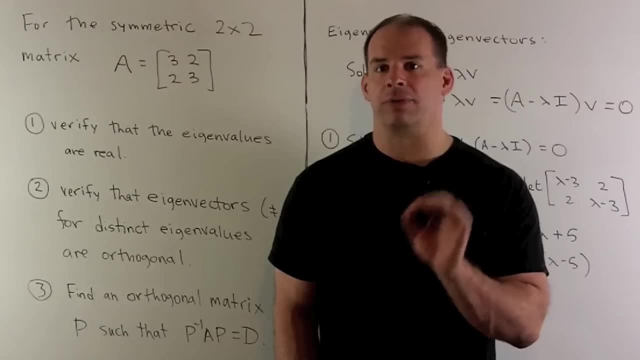 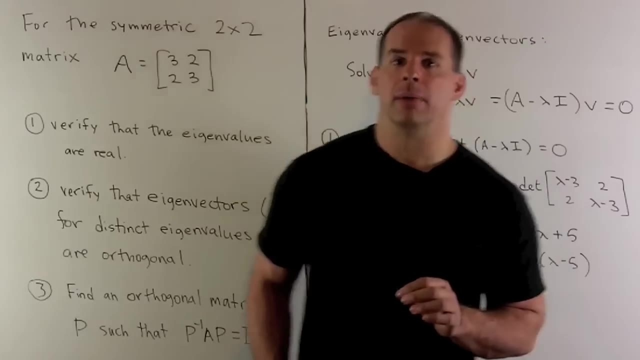 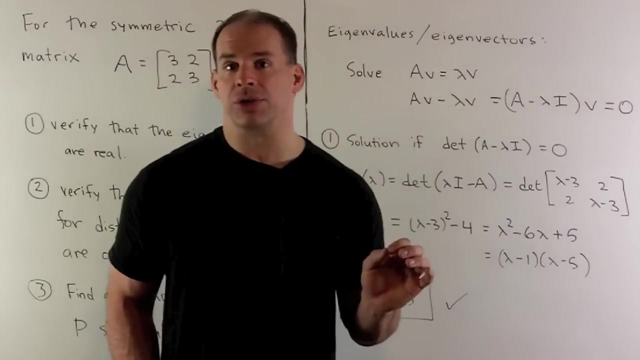 a real symmetric matrix. we can always put it into diagonal form using an orthogonal matrix. Okay, step one: to verify that the eigenvalues are real. So let's just go through our process for finding eigenvalues. We start with the equation: Okay, we're going to take our matrix A, multiply it by a vector. 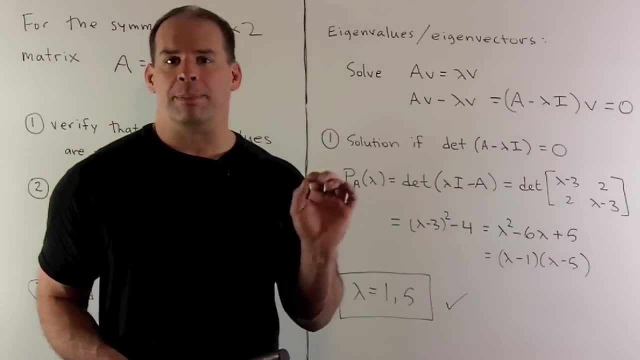 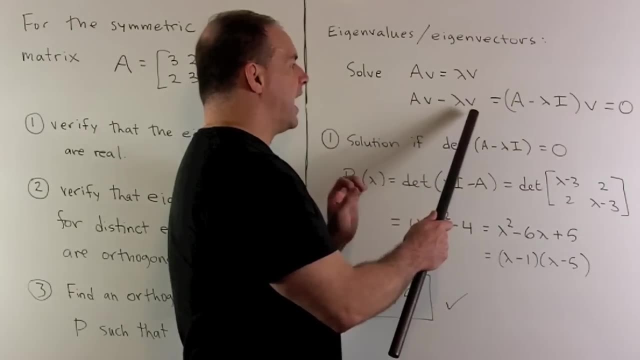 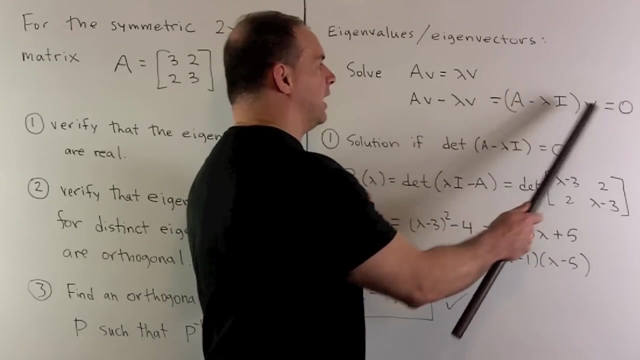 V. If I have V as an eigenvector, what we get back is some scalar lambda times V. I push the lambda V to the other side. Then I can factor out A minus lambda I times V. So the idea here is: lambda I times V is just equal to lambda V. Then we set that equal to zero. 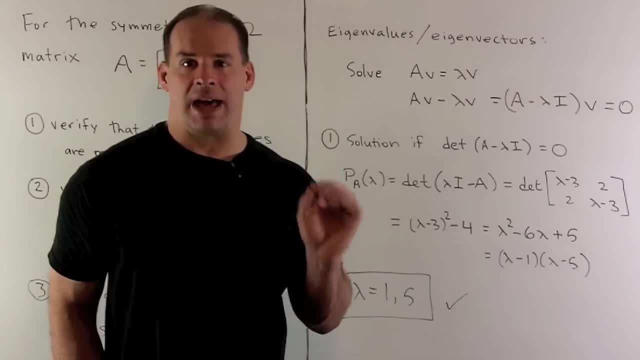 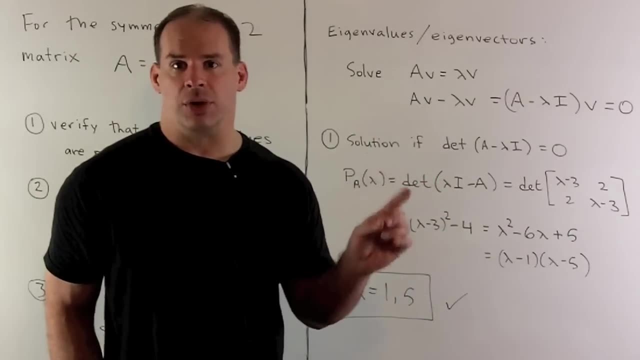 So we're just trying to find out what the eigenvalues are. So we're going to take our matrix A and we're going to find the null space of A minus lambda I. Now that's going to have a null space if, and only if, the determinant of A minus lambda I is equal to zero. So 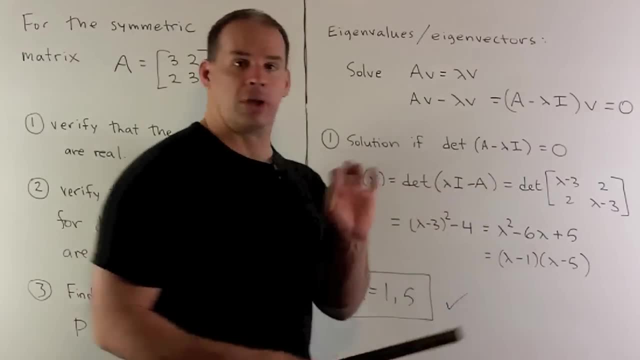 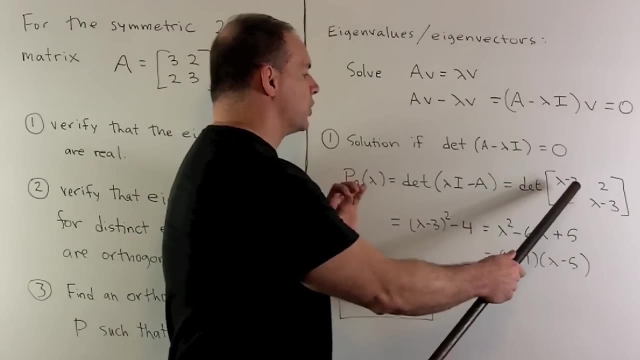 we're going to call that expression Okay, and I'll just switch the order here. Okay, it's only multiplying by minus one. We're going to call that our characteristic polynomial. So if we work that out, this is going to be equal to zero, exactly when lambda is equal. 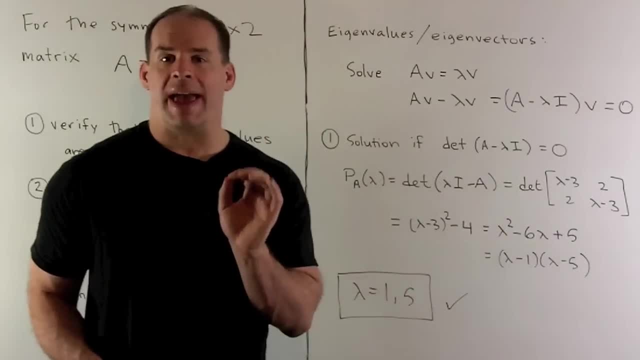 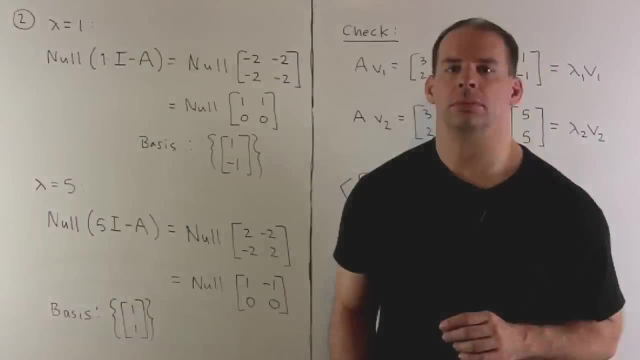 to one, or lambda is equal to five. So my eigenvalues are one and five. So I'm going to have my eigenvalues equal to one and five and that verifies that the eigenvalues of my real symmetric matrix are real. Now we want to find a basis of eigenvectors for our 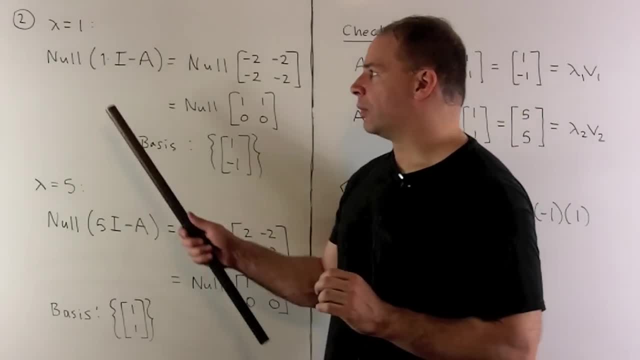 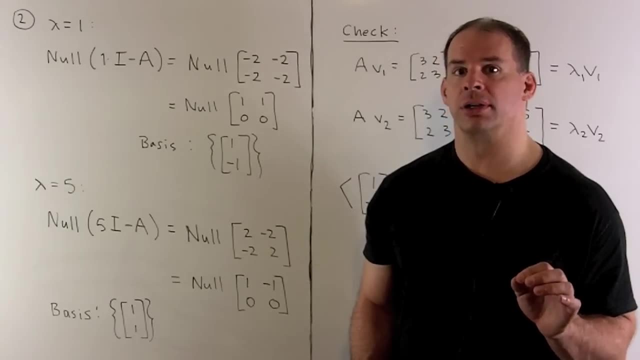 matrix A. So here, for each eigenvalue we're going to find the null space of lambda I minus A. That'll give us our space of eigenvectors. Now, for lambda equal to one, we have null of one times I minus A. So again, I can't even use my vector, So I'm just going to. 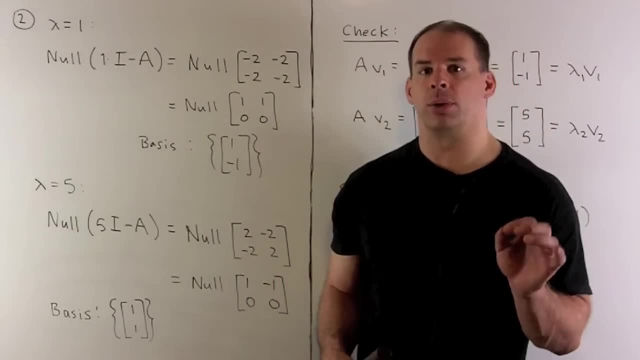 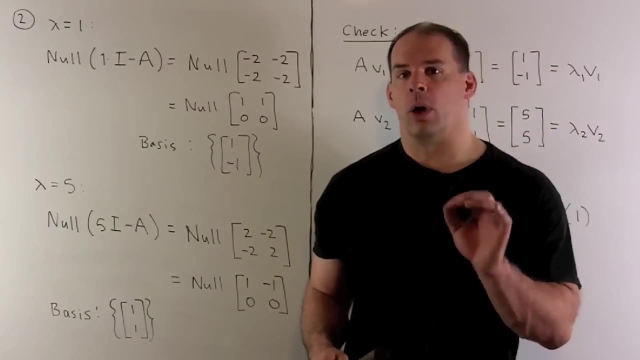 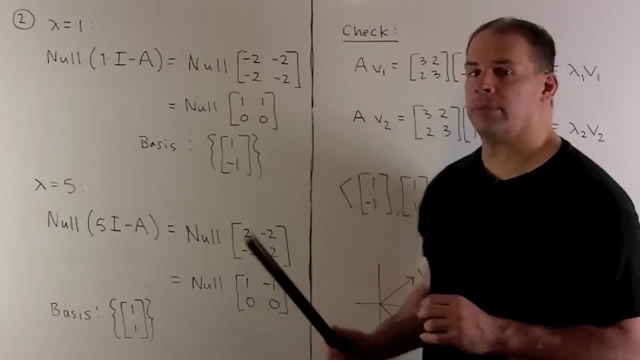 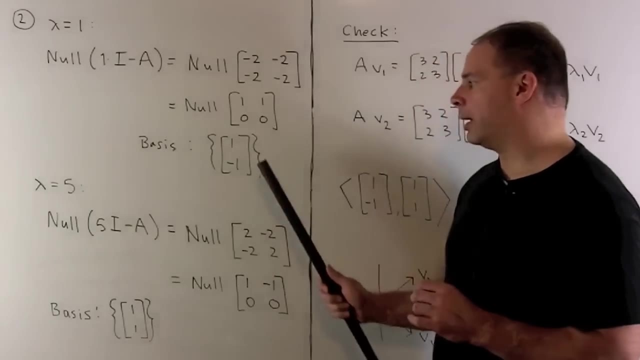 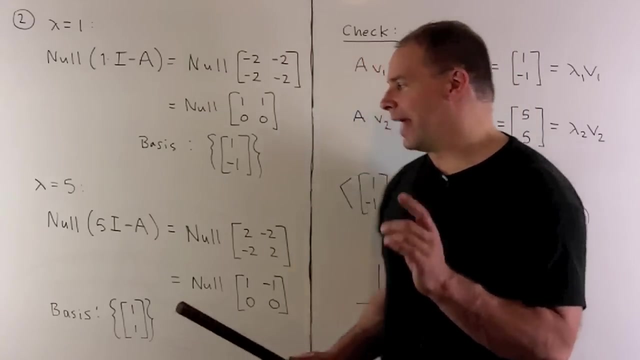 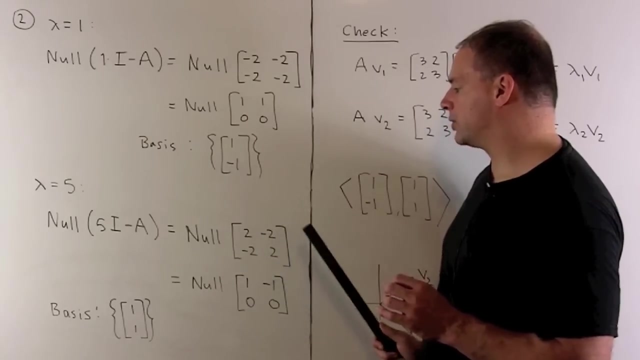 going to be given by the vector 1, minus 1.. So our space of eigenvectors with eigenvalue 1 is given by the span of 1, minus 1.. If I let lambda be equal to 5, then we're looking for the null space 5i minus a, or the null space of 2, minus 2, minus 2, 2.. 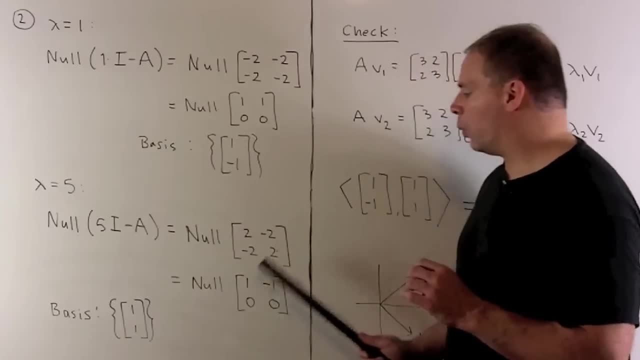 We row reduce, Then I'm looking at 1, minus 1, 0, 0.. Then here a basis for the null space is going to be 1, minus 1, 0, 0.. Then here a basis for the null space is going to be 1, minus 1, 0, 0.. 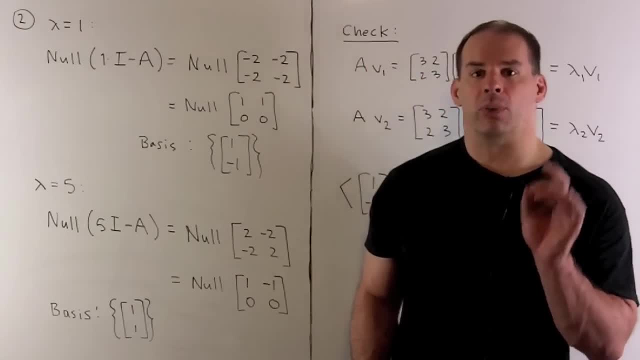 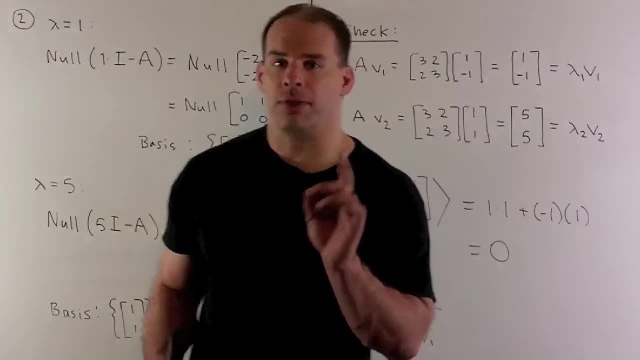 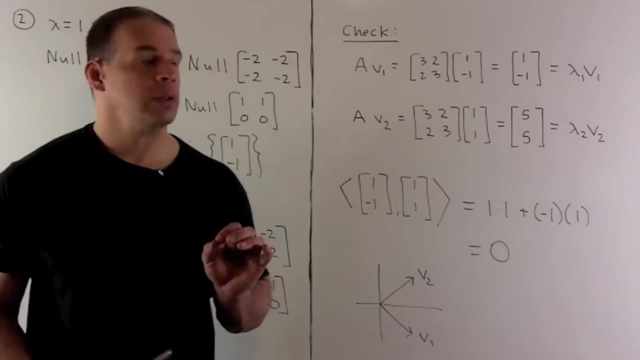 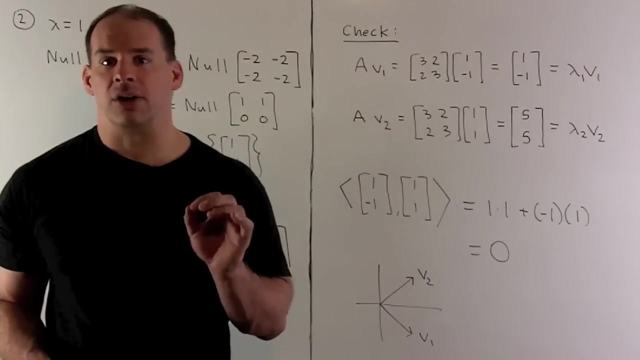 So we have our basis of eigenvectors. Now there's a few things we want to check. First, I want to apply A to each basis vector, just to verify that we have eigenvectors. So if I apply A to our first vector 1-1, what comes out is the vector 1-1. 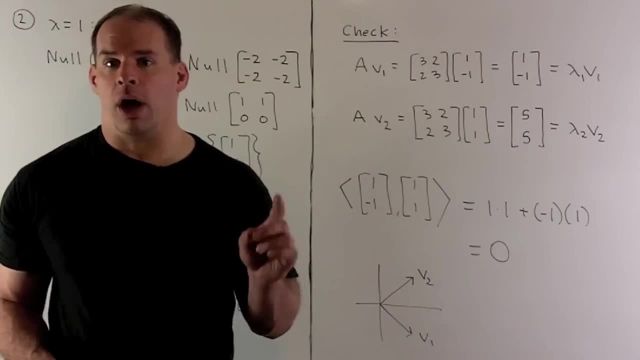 So in this case the eigenvalue is equal to 1.. So what's coming out is lambda times our original thing. So that checks out For our second vector 1-1,. we apply A. What comes out is going to be the vector 5-5.. 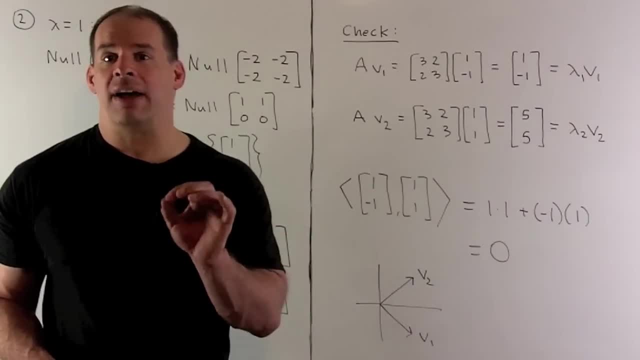 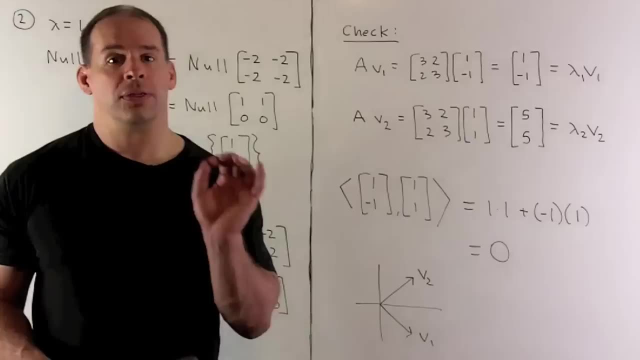 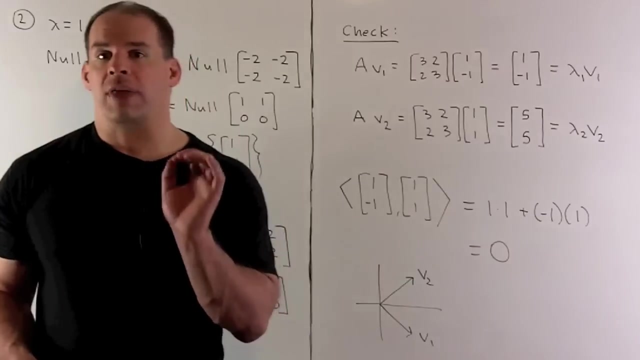 If I factor out a 5, we have our eigenvalue 5 times our original vector. So that checks out also. Third thing we want to check: I want to see that the basis vectors are orthogonal with respect to the usual inner product. 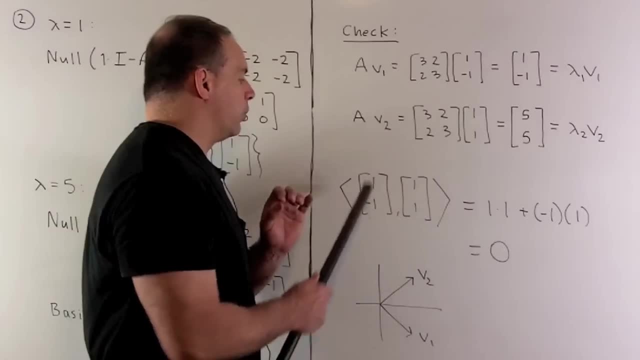 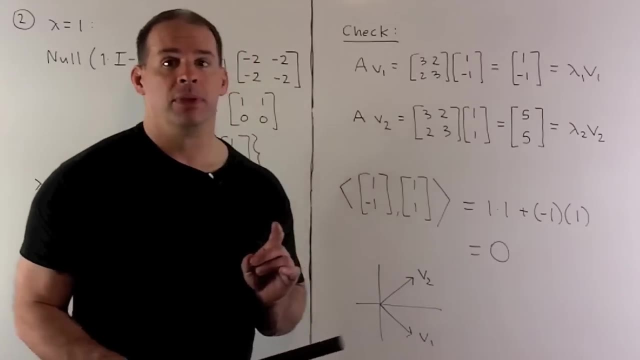 So if we compute that, we're taking 1-1 against 1-1.. So I'm just going to multiply across, take the sum and see what comes out. So here I'm going to have 1-1.. So I get a 0.. 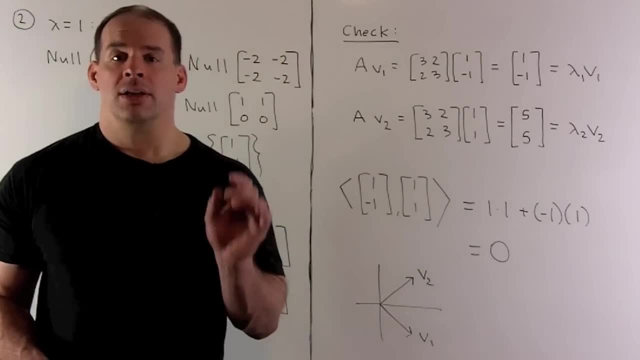 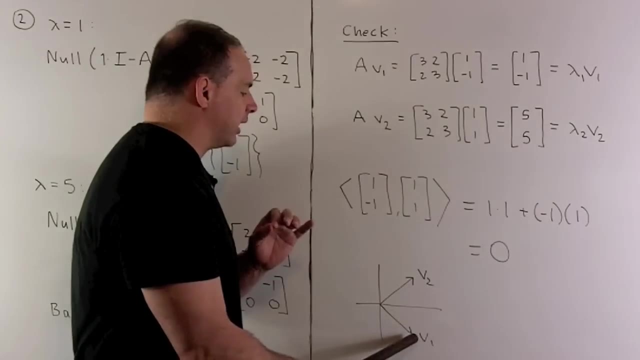 And then that means our vectors are orthogonal. Since we're in two dimensions, that means perpendicular, So I'm going to multiply. So if we were to actually draw these vectors, we'll have V-1 pointing down like this along a 45-degree angle: 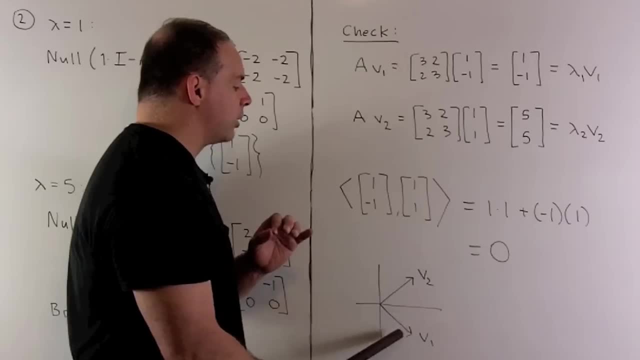 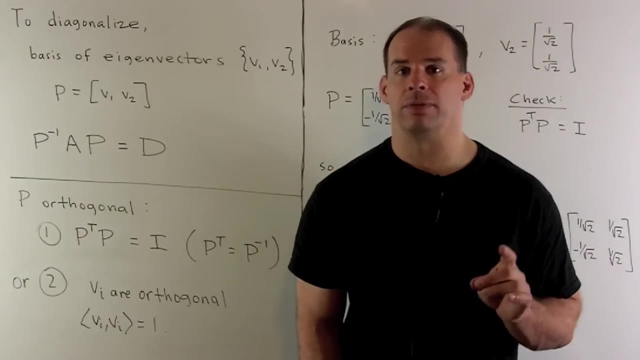 1-1 points up along a 45-degree angle, So the angle between them is 90 degrees, So they're definitely perpendicular. To put our matrix A in diagonal form, we need to set up our change of basis matrix P. 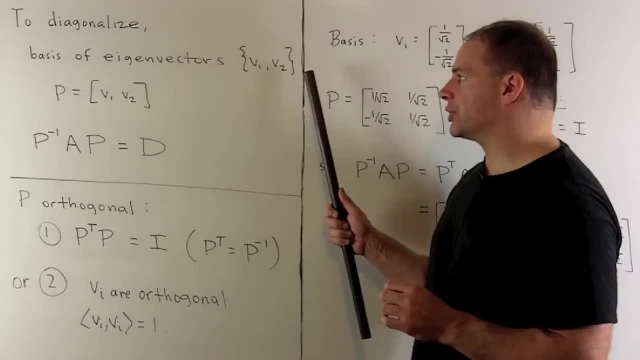 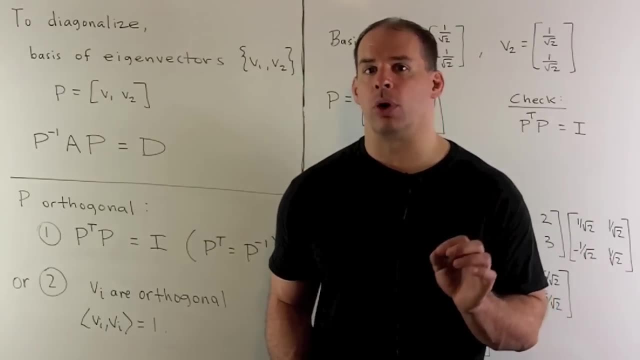 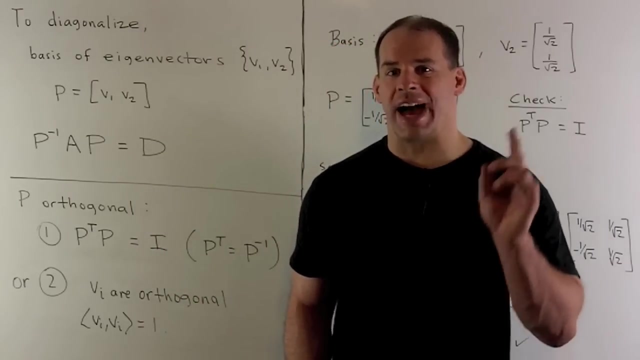 To do that, we take our basis of eigenvectors, We load them in as the columns of P. Then the equation that puts this in diagonal form is going to be P inverse A. P is equal to D, where D is a diagonal matrix whose diagonal entries are just our eigenvalues, in the same order that we've loaded them in as our basis vectors. 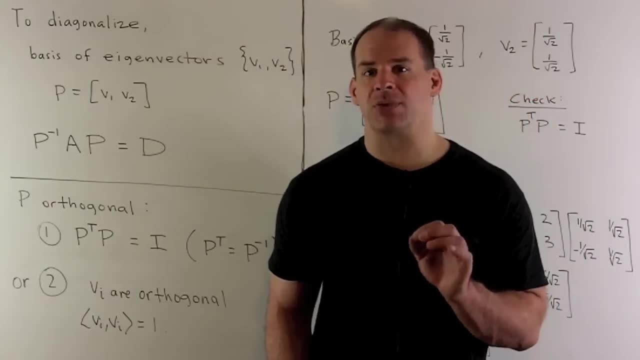 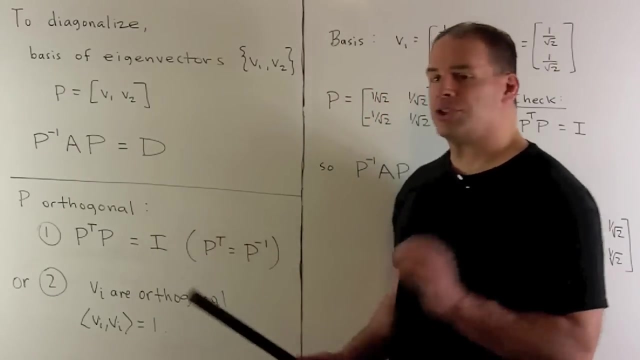 Now a question asks for a little bit more than this. We also want that our change of basis matrix P is orthogonal. So that's just going to mean if I take P transpose times P, I get out the identity matrix. So another way to say that is that P transpose equals P inverse. 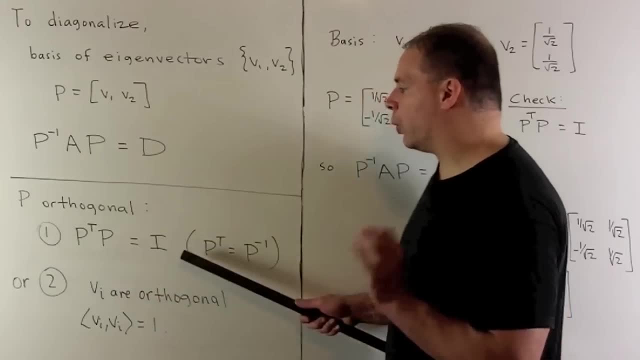 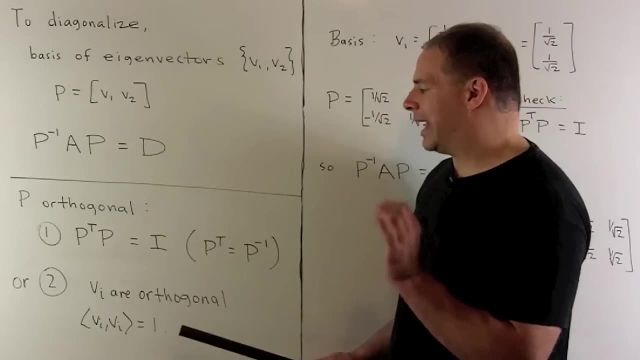 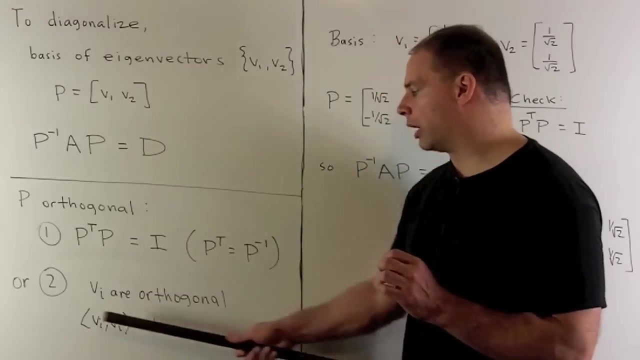 And if we unpack all the equations in one, so if you take each row times column multiplication, what's going to come out is that we have each of our basis vectors orthogonal, And if we take the length of each basis vector, we get 1.. 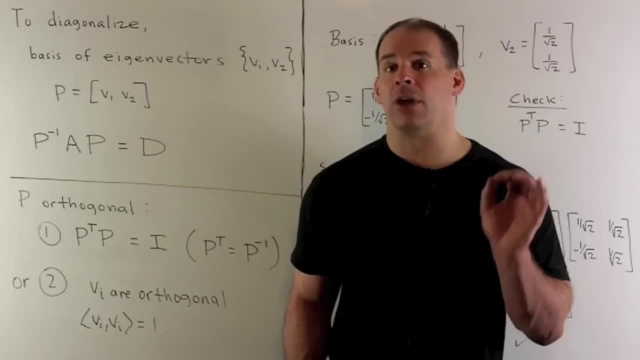 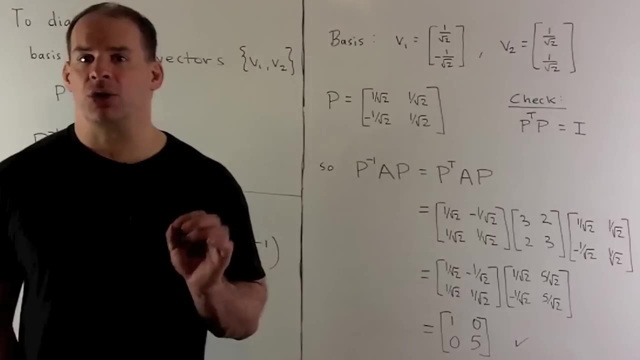 So our basis vectors are mutually orthogonal And they're unit vectors. Now, in our special case, we're almost there: We have our basis vectors orthogonal, but we don't have unit. So we just need to compute the length of each basis vector and then divide. 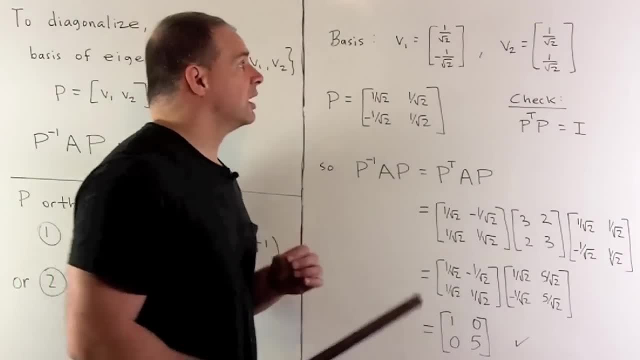 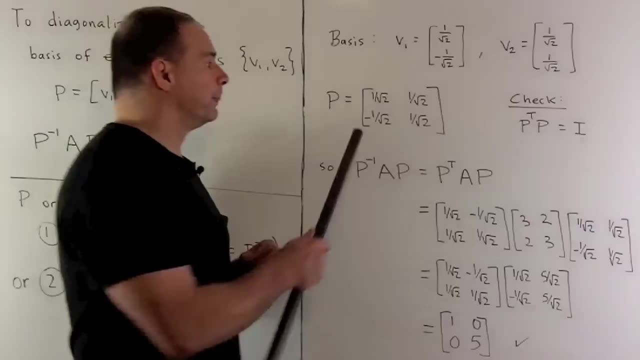 So the basis that we're going to use, our orthonormal basis, is going to be given as so. Now I set up my matrix P. Okay, you want to check that P transpose times. P is equal to your identity matrix. 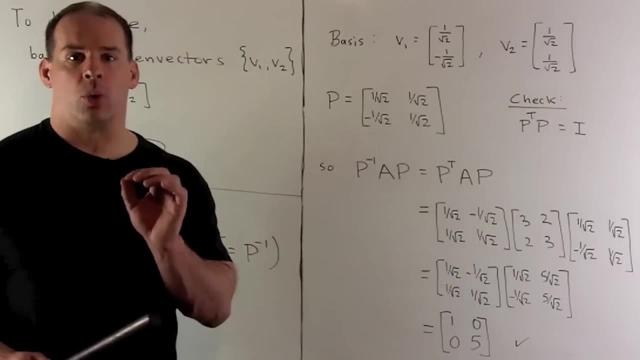 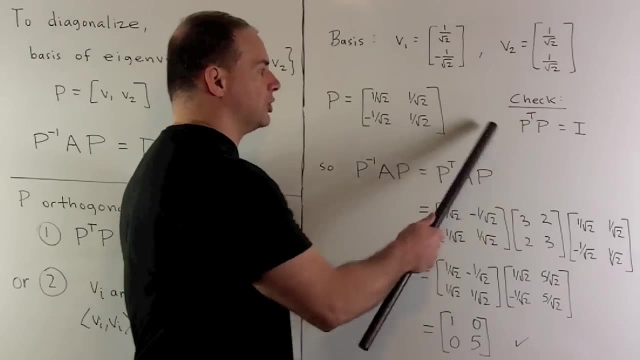 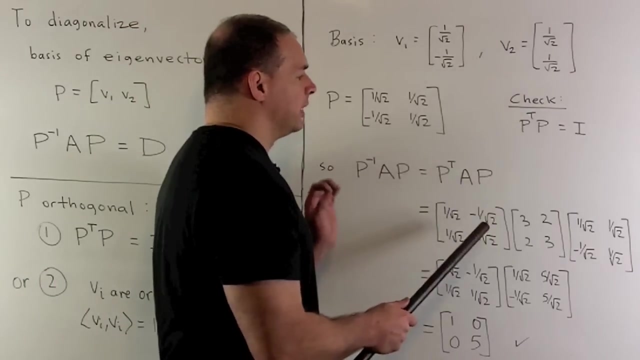 And then we just set up our equation. So I take P inverse AP Note, I'm allowed to use that P inverse is equal to P transpose. Okay, if we just check that, Then I work out my multiplication. Now you'll note A times P is going to be A times eigenvector 1 times eigenvector 2.. 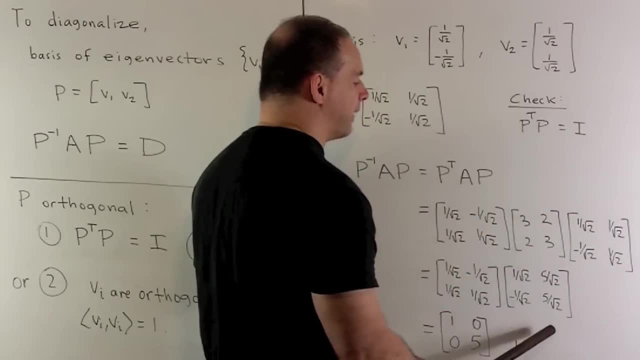 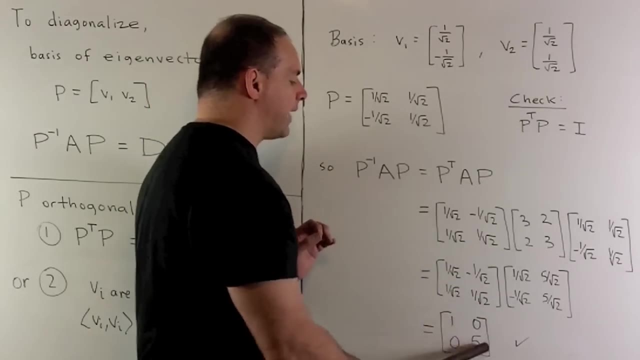 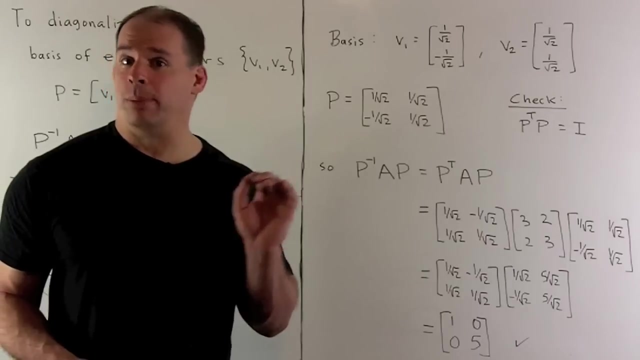 So I just multiply here by a 1 in that column, this one by a 5. Multiply by P, transpose, And then that's going to get me to 1, 0,, 0,, 5.. So we have that. our matrix A can be put in diagonal form using an orthogonal matrix. 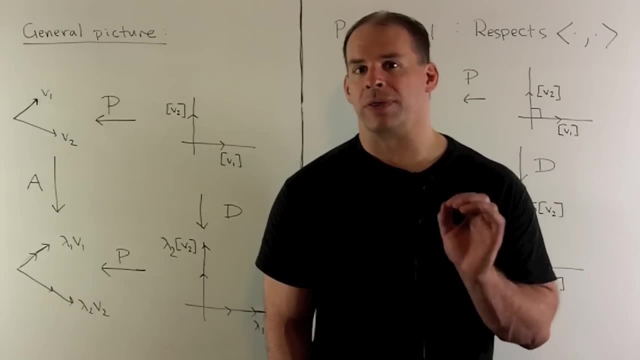 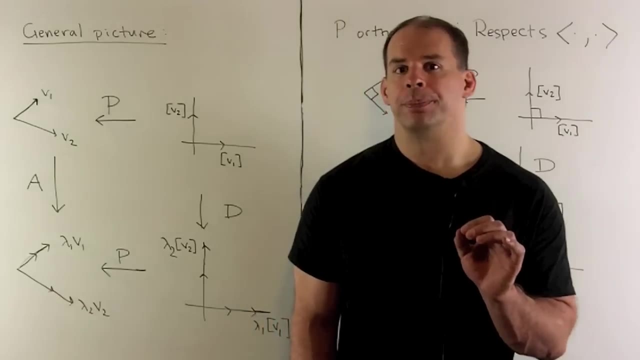 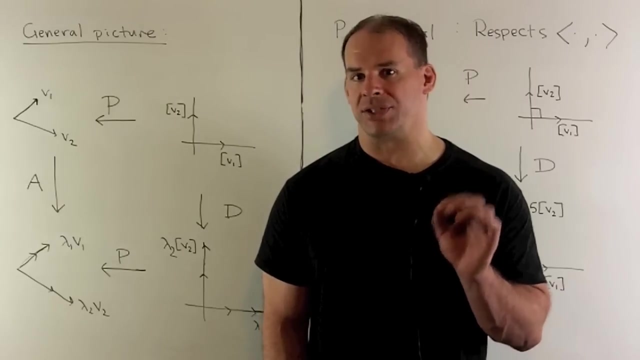 So the big question is: what do we get for using an orthogonal change of basis matrix? We'll have two answers to that. First answer: if I'm interested in this business of diagonalizing matrices, at some point I have to take the inverse of the change of basis matrix. 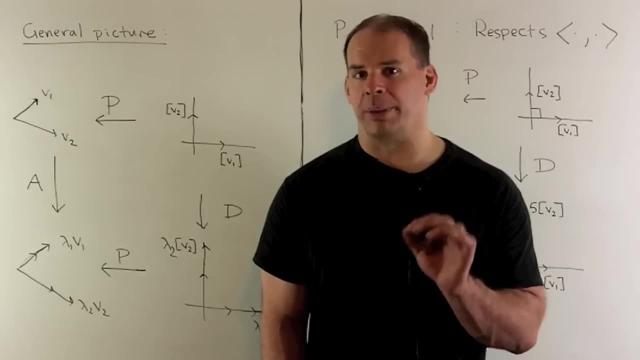 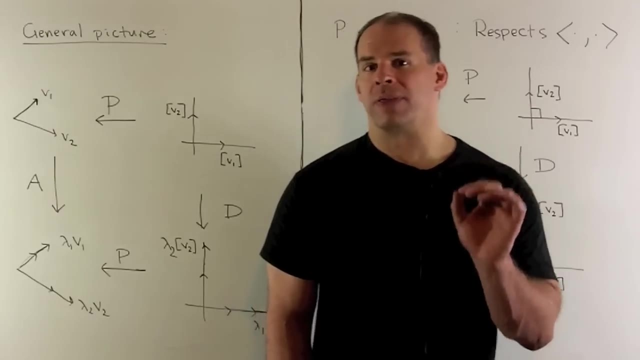 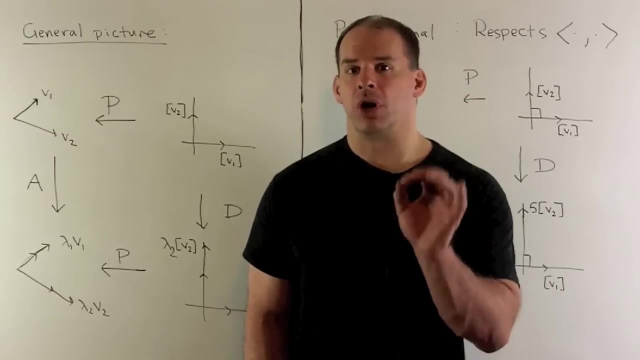 So if I have an orthogonal change of basis matrix, we get the inverse for free. We just take the transpose. So having an orthogonal change of basis matrix can cut back on our work. For the second answer, first let's review what's happening when we diagonalize a matrix. 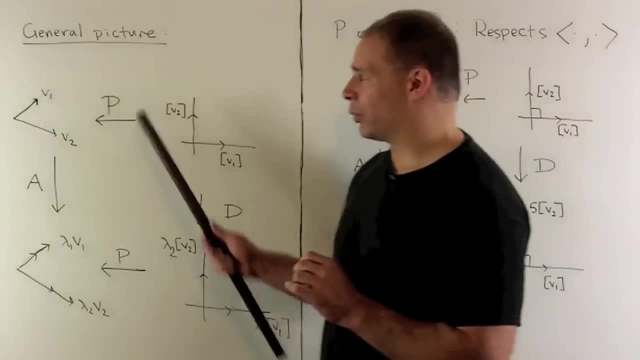 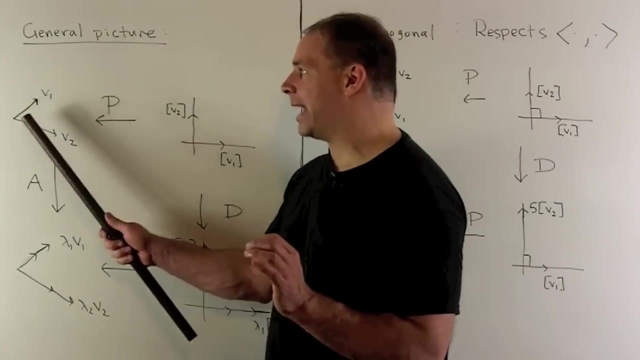 Now for a picture, say in: Okay, we're doing the plane. I'll just have a basis of two eigenvectors. What we're going to do is, when I apply my matrix A, I'm just going to stretch each eigenvector out by its eigenvalue. 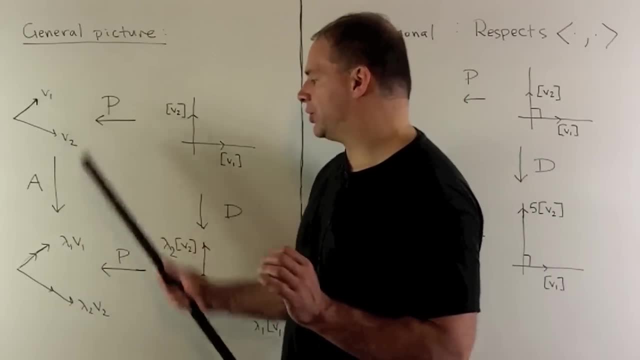 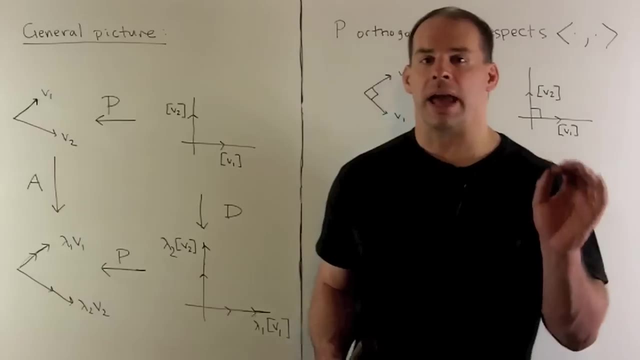 So V1 goes to lambda 1- V1.. V2 goes to lambda 2- V2.. So the directions are the same. We're just doing some rescaling. Now, when I change over to coordinates for the eigenvectors: okay for my eigenvector basis. 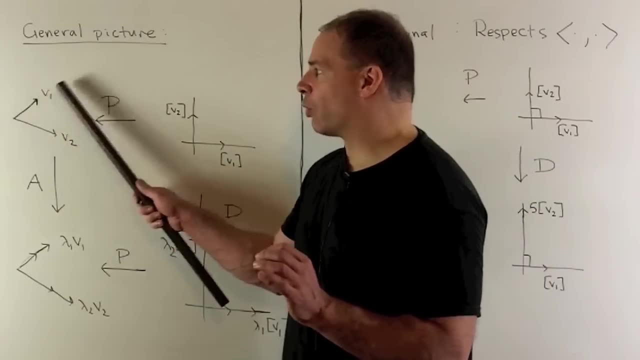 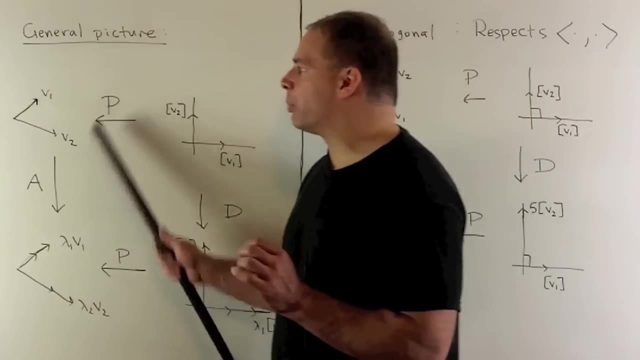 well, things over here might not be okay at right angles, but when I go to coordinates they will be at right angles. So you'll note if we were caring about an inner product on this side, we just did some damage to it by moving over to here. 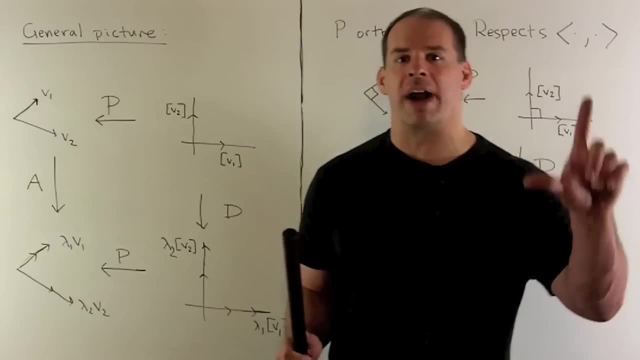 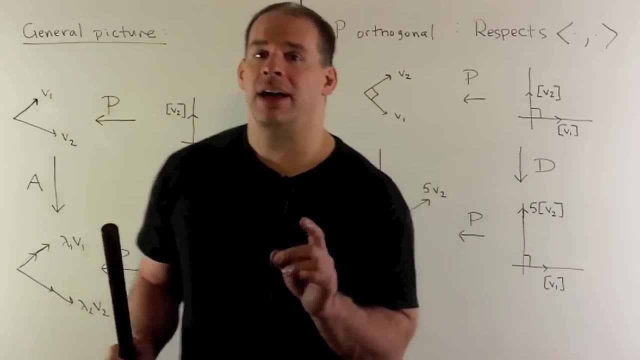 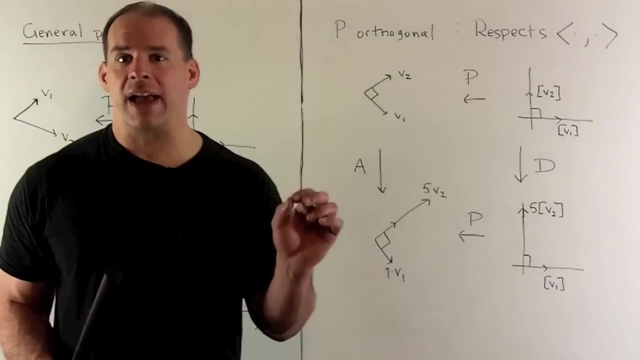 Okay, because if we were respecting the inner product, then we'd want right angles to go to right angles- Not happening here. Okay, if I have an orthogonal matrix, then it's going to preserve the inner product, which means right angles go to right angles. 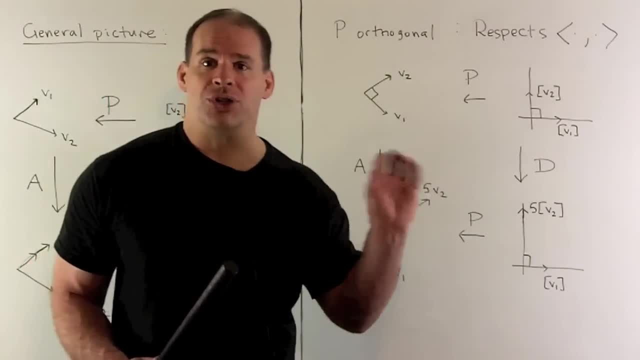 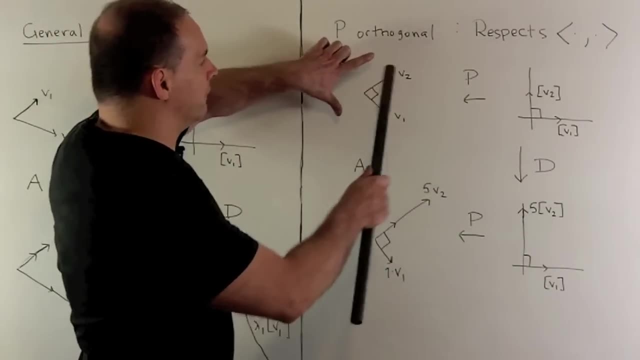 Things of a given length go to vectors of the same length. So for instance here: okay, in the situation we were looking at, okay, we have our unit vectors here. When I go over to coordinates, they're going to stay unit vectors. 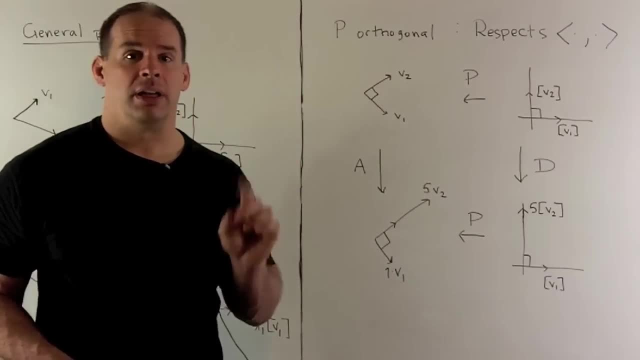 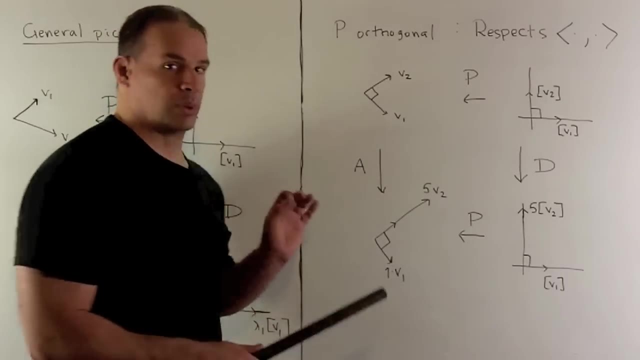 and they're going to stay at right angles If I apply my symmetric matrix A. okay, these are eigenvectors, so we just stretch out V1 by 1, which means we leave it alone. For V2, we stretch it out by 5.. 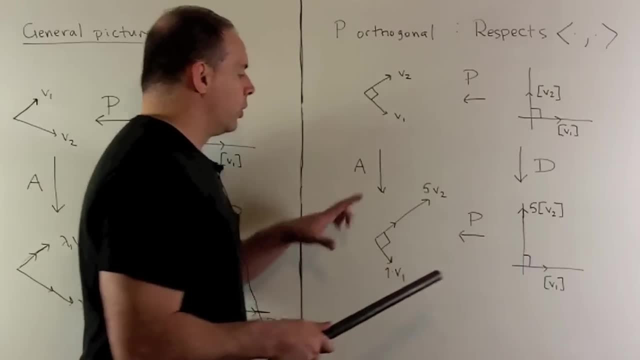 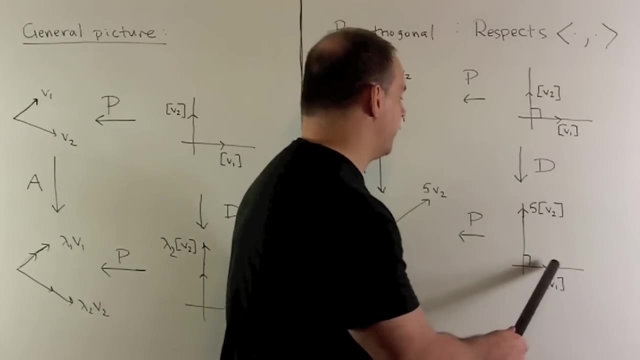 Now, when I push this over to coordinates, well, the idea is, if I just take these two vectors here, pick it up, it's going to sit exactly on top of these two vectors here, So we're not distorting the inner product at all. 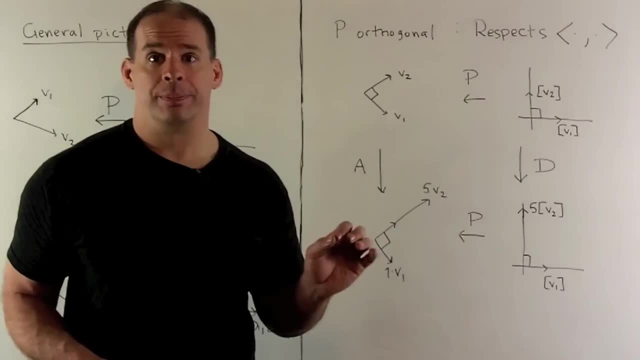 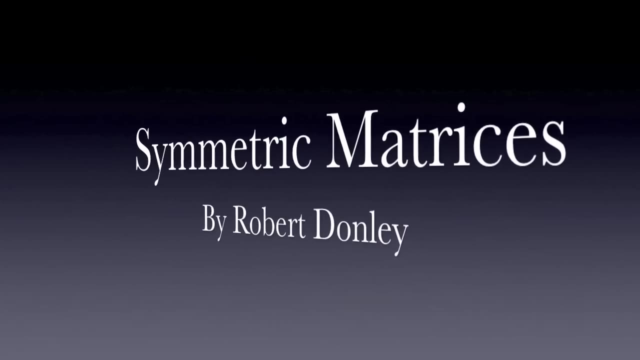 Right angles go to right angles. Lengths are preserved. That's going to be really useful in some applications. Thank you, Thank you. 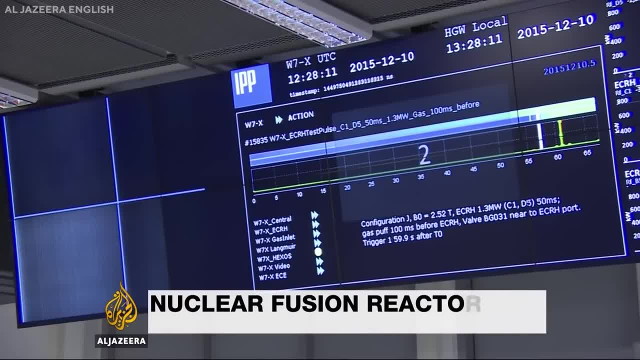 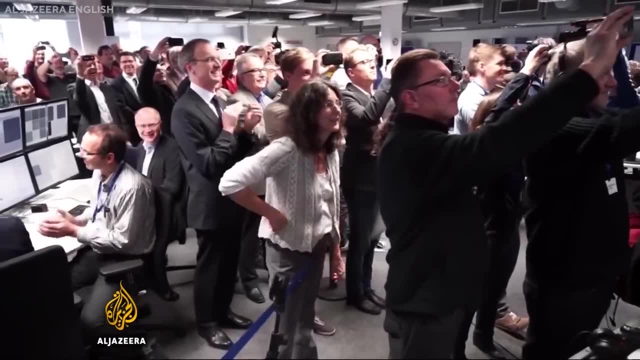 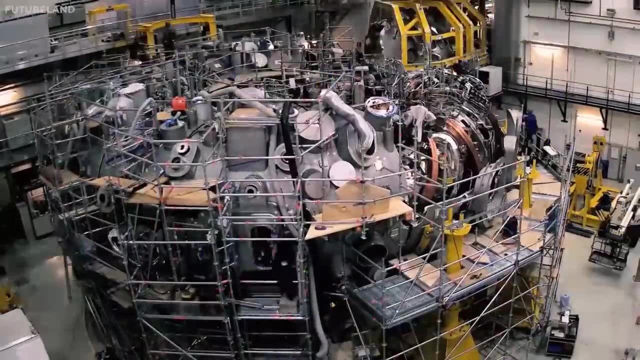 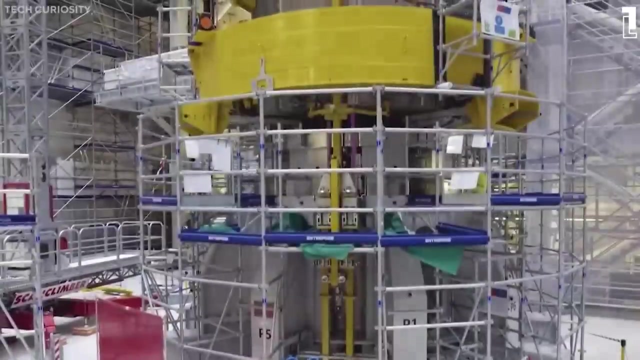 In construction. it's time to fire up Germany's revolutionary fusion machine. It's a tense moment. Welcome to a groundbreaking moment in the world of nuclear fusion. Germany's latest marvel, a cutting-edge nuclear reactor, is finally kicking into gear, promising to outshine even the International Thermonuclear Experimental Reactor. 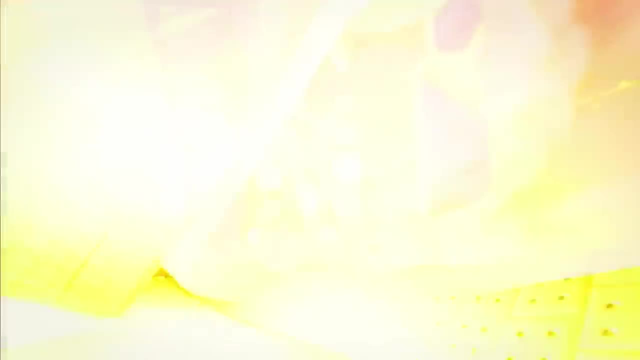 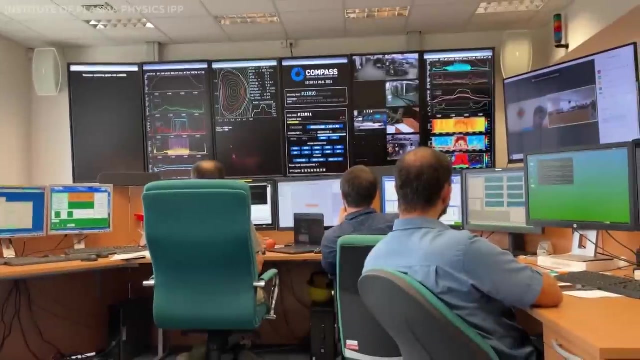 IHAR in its quest for clean, limitless energy. This reactor isn't just a leap forward. it's a quantum jump in the technology that could power our future. Stay tuned as we dive deep into how Germany is leading the charge, potentially revolutionizing our energy landscape forever. 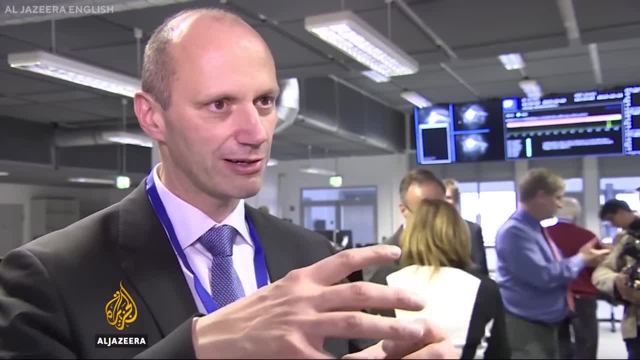 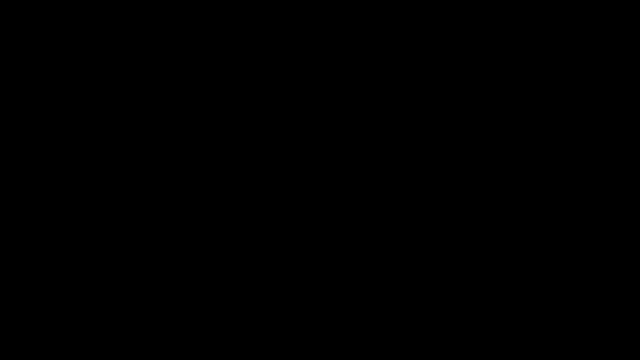 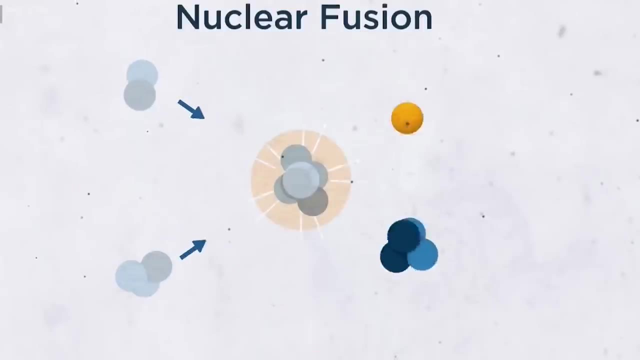 If we achieve everything to put all the elements together to make fusion happen, then we have an abundant, clean, CO2-neutral, climate-neutral energy source. Nuclear fusion is the process of combining lighter nuclei into heavier ones, releasing enormous amounts of energy in the process.